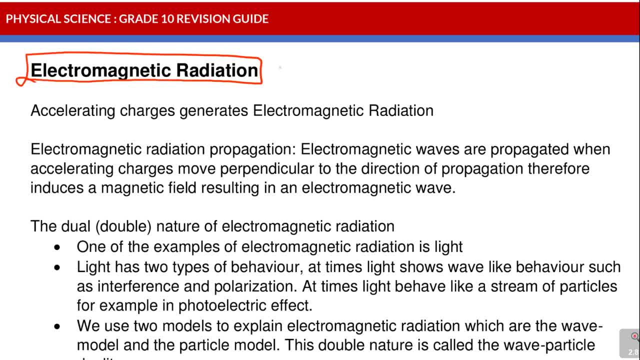 actually, what is it? what is electromagnetic radiation? or how is it formed? or propagated? that's the word they use. how is it propagated? sometimes it's a simple answer. they need to say electromagnetic charge. so what is it? accelerating charges? that's it. accelerating charges generate what electromagnetic radiation? or the question, as you say they will say, how is it generated? you just say: 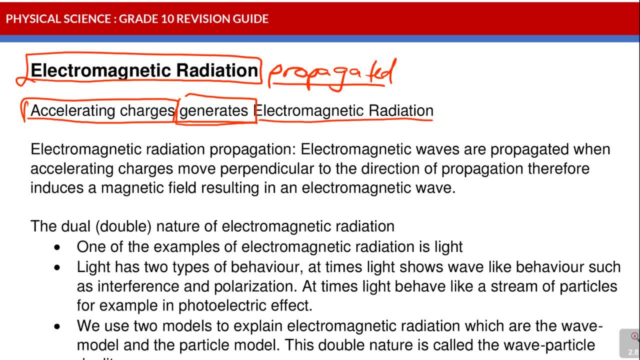 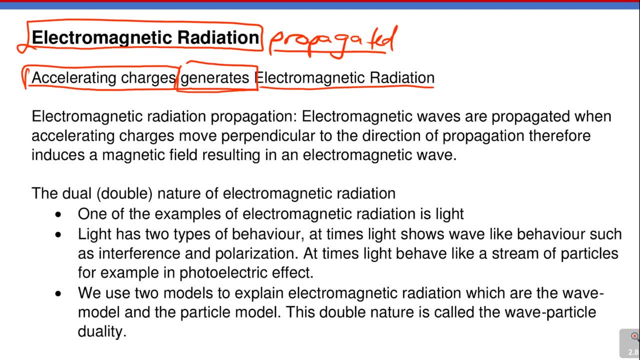 by the accelerating charges. so as these charges are accelerating, electromagnetic radiation is propagated. all right, so now, electromagnetic radiation propagation- again an important statement you need for your exam. what i say says: electromagnetic waves are propagated when accelerating charges move perpendicular to the direction of propagation, therefore induces a. 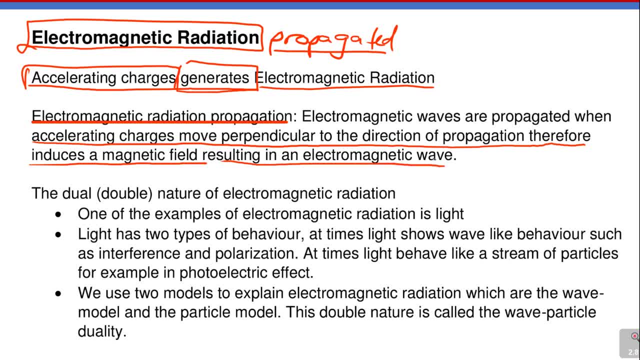 magnetic field, resulting in an electromagnetic wave, actually is the perpendicular between the electric field and the magnetic field. so, as these also are changed, i'll say: this is the electric field and this is the magnetic field. so they are at 90 degrees perpendicular to each other. as these: 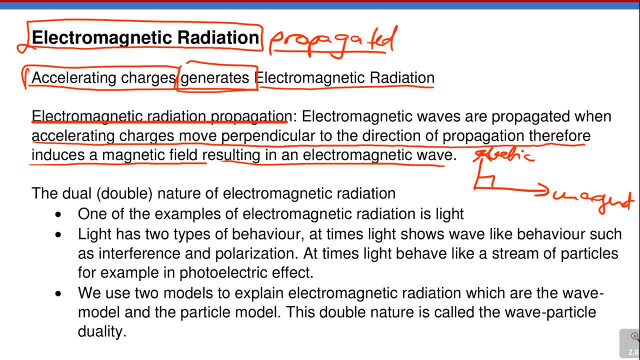 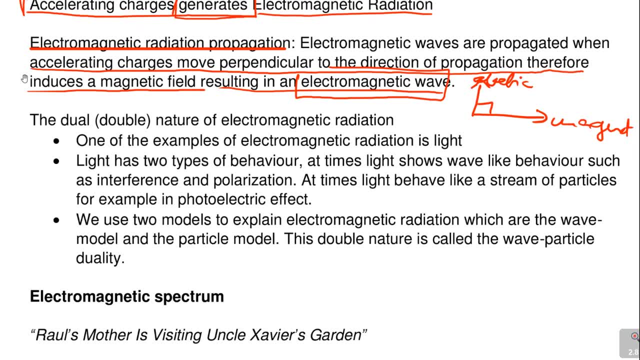 are oscillate between electric and magnetic field, and electromagnetic radiation is produced. now the next part we are going to look at is for you to understand the dual nature of electromagnetic radiation. dual means double, double nature. so one of the examples of electromagnetic radiation is light, the light that you see every day. so light has two types of. 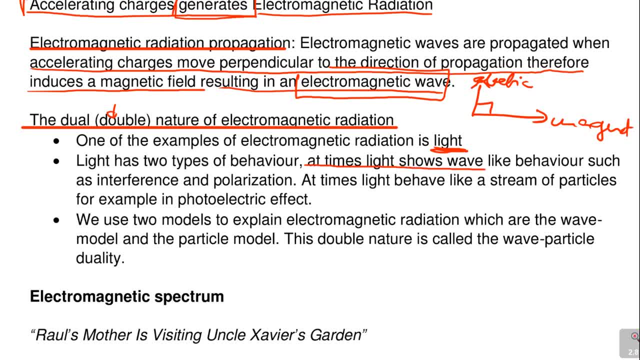 behavior. at times light shows to behave like a wave, so light shows a wave-like behavior. for example, what are the wave-like behavior in light? there is interference, remember constructive interference, destructive interference, such uh, such as superposition is another word- and then and polarization. that is the wave-like behavior of light, so it can show those characteristics. 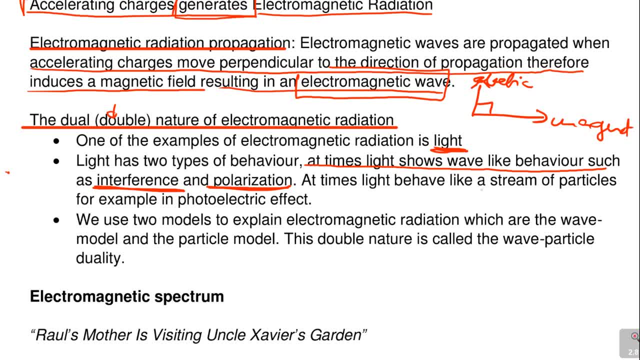 at the same time, light behaves like a stream of particles, for example in photoelectric effect, which are going to land at a later stage in bread 12. so the fact that light can have this type of two behaviors: it can behave like a wave and then it can behave like a stream of particles. this is 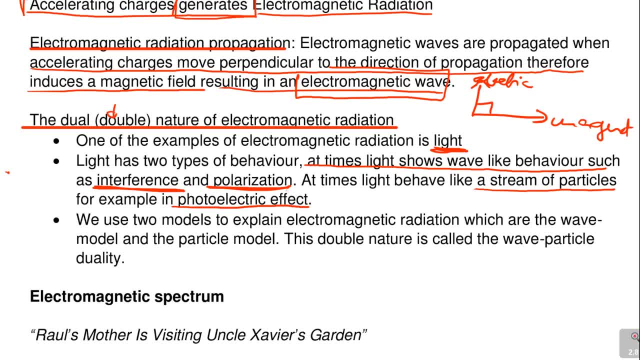 called the dual nature. that's what light shows. to behave like a stream of particles makes electromagnetic radiation unique. unlike the waves we did looked at the mechanical wave, which is the transverse and the longitudinal wave, now this electromagnetic wave has got a double nature, which is ppf, like a wave. at the same time, it has also a behavior of as if it. 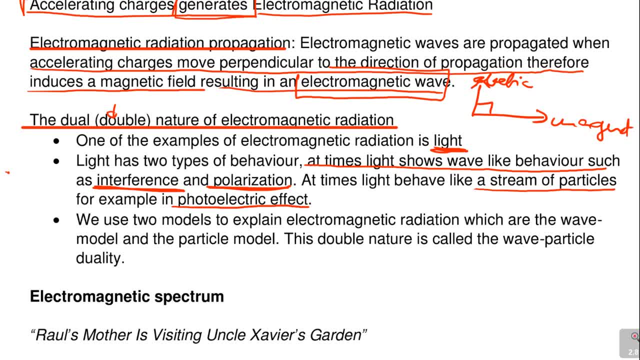 is a stream of particles. now we use two models to explain electromagnetic radiation, and the electromagnetic radiation is a stream of particles. it is a stream of particles. it is a stream of particles and what is the model? the first model is called the wave model, where we look at it when it's. 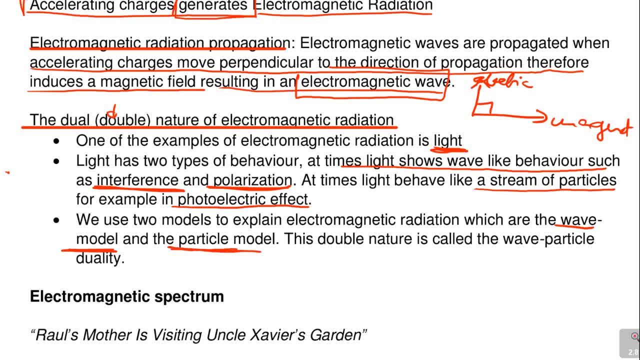 behaving like a wave, and then we've got the particle model, when light starts behaving like a particle. now this double nature is called the wave particle duality. so whenever you listen to or you start reading about electromagnetic radiation, you'll be introduced to this term wave particle duality, meaning it behaves like a wave and then you start reading about electromagnetic 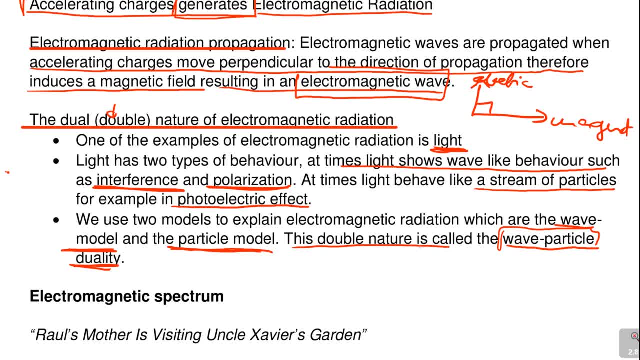 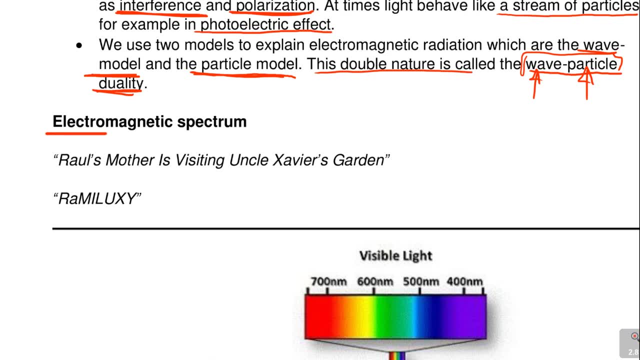 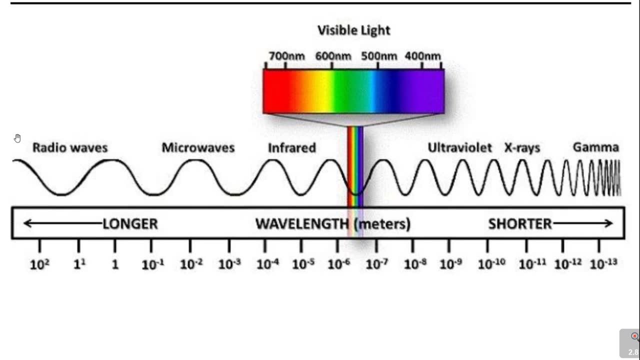 radiationム. now the next important one is the electromagnetic spectrum. this is- they will expect you to know- the arrangement of the electromagnetic wave in um. in order of what? increasing frequency or in order of decreasing wavelength. so look at it. this is the arrangement, and in here you can see that. 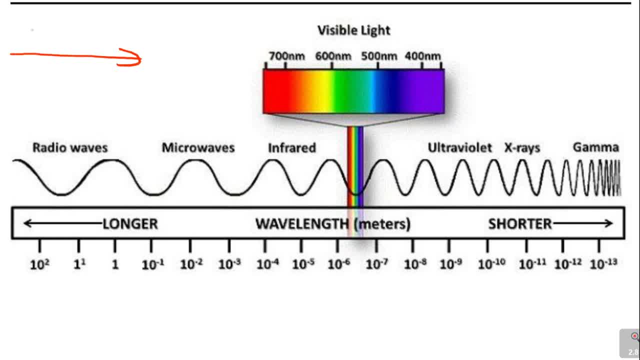 frequency is increasing this direction. this is increasing what? increasing frequency. but don't forget, as frequency is increasing, the wavelength will decrease. it's the opposite. and then, with increasing frequency, you can also look at this, this direction. when frequency is increasing, this is the increase in penetrating ability. penetrating ability. 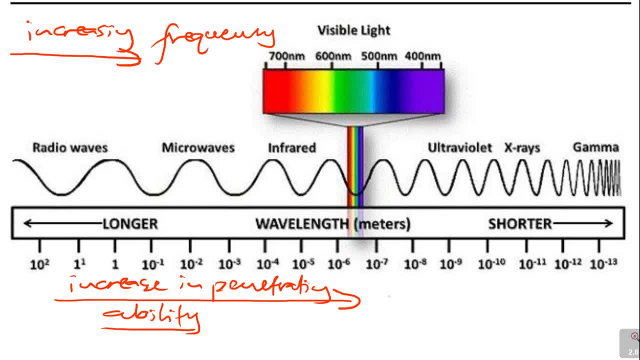 so the ability of the waves to penetrate, or increasing energy. so what do you mean? obviously radio waves. at the beginning it means they have low energy. gamma rays are high energy or high penetrating rays. so these are the two extremes. if i give you radio waves, these are: 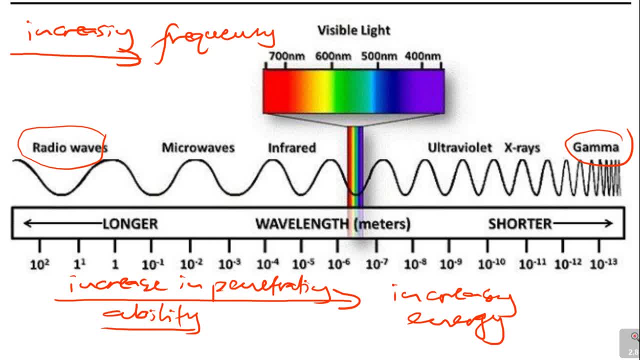 low. actually, they are not even penetrating. these are low frequency waves, gamma rays, high frequency, high penetrating waves. so how do you simple master this? uh, what do you use? if ever you want to master this? i just want to uh in my mind, i just want to in your mind. actually, i wanna impress this, or to 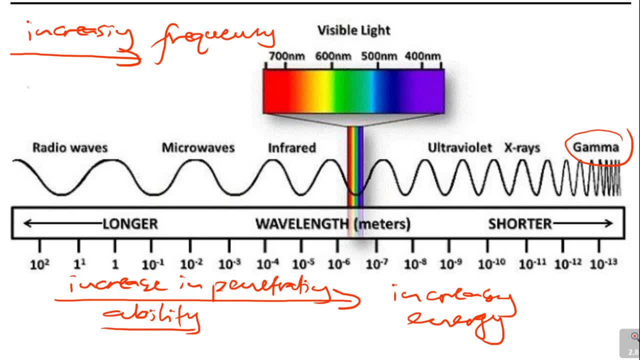 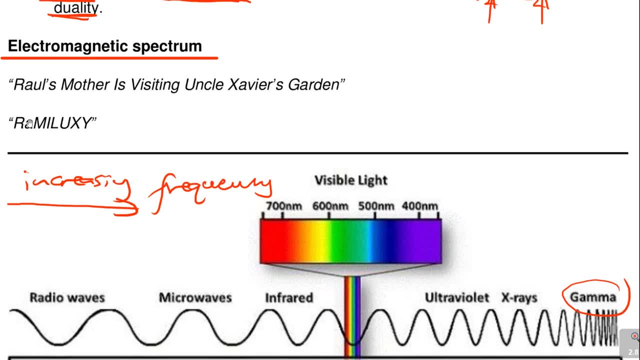 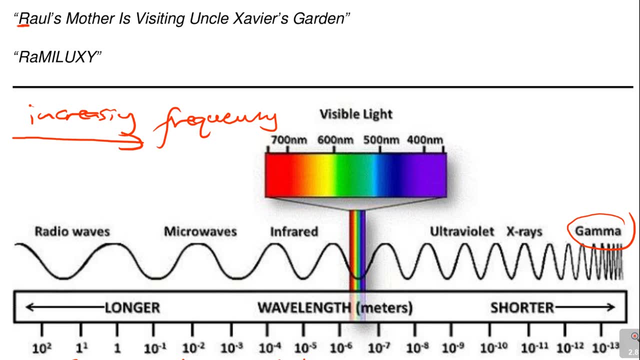 just stick this to your mind. you don't need to sometimes claim these are words. sometimes they come with this. you see, like here raoul's mother is visiting uncle xavier's garden or ramilaxi. you can do that, you can use this. where r is the radio waves there? look at, these are the radio waves m is. 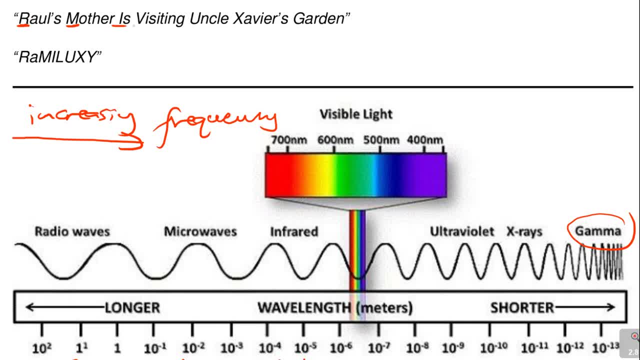 the uh microwaves. i is the interaction of radio waves and xavius. you can use this on radio waves. the power of radio waves is the radio waves, m is the microwaves, i m is the efficiency of the radio waves. the infrared V is the visible light, U is the ultraviolet, X is the x-rays and G is the. 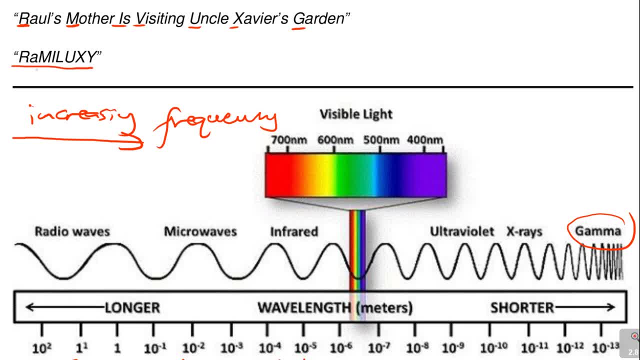 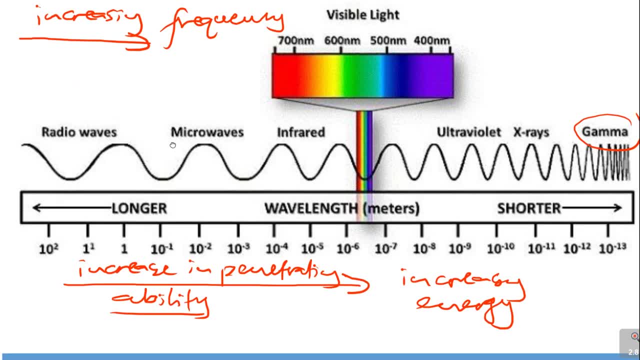 gamma rays, Or Ramilaxi is the same: R radio wave, M, microwave, I, L, U, X, Y- Still fine, but what do I use? I prefer to be able to do this. What if I forget this statement altogether? So 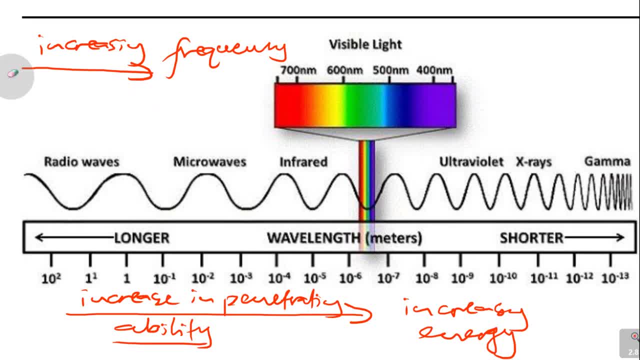 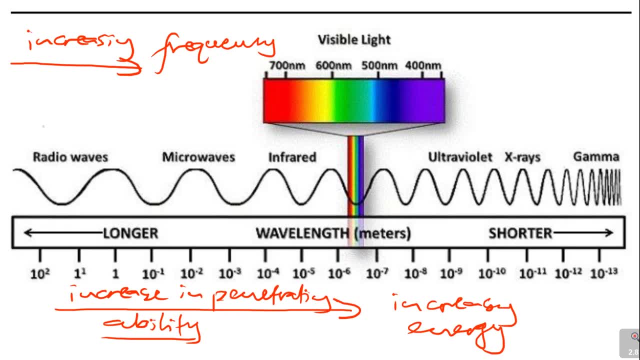 what do I do? I try to put some images in my mind concerning these waves. The first one I will say is: what is the most important gadget that you always have? Always, It's a. what It's? a cell phone. These days, you can't do without a cell phone. I mean your WhatsApp and everything is. 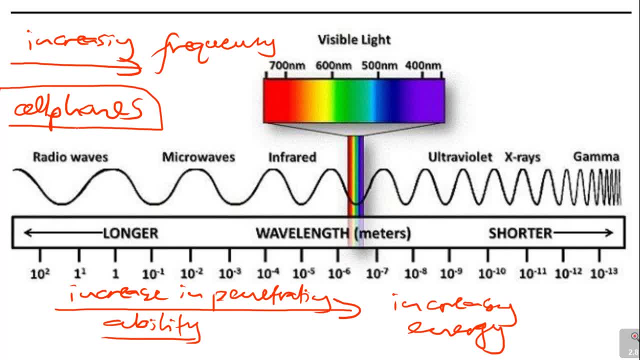 in your cell phone. Now, in your cell phone, what are you going to use to listen to your FM radio? with your earphones? You use radio waves, So you start there. The most important gadget currently is your cell phone that you can use every day. That's where you get your radio waves, Are you? 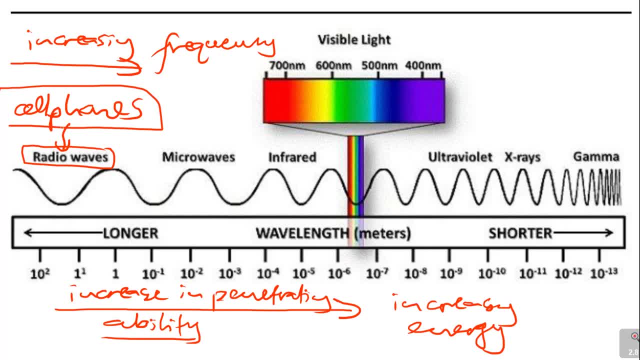 with me. And then, once you know the first one, the most dangerous waves that you never want to come across is the end. Gamma rays, Very dangerous. These you like, you know. you always remind yourself what is the safest one? Radio, What is the last one? Gamma, Radio, gamma. Once you, 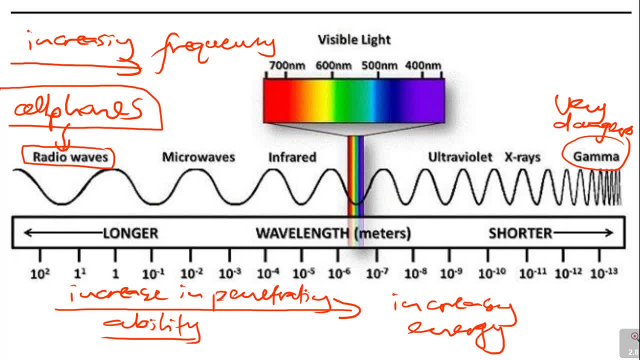 master these in between, then you can play around also. After that you're saying, okay, I've got my cell phone in my hand and I know the dangerous ones. I'll never have to come across as the gamma rays You say when I go into my house or into- uh, into your. 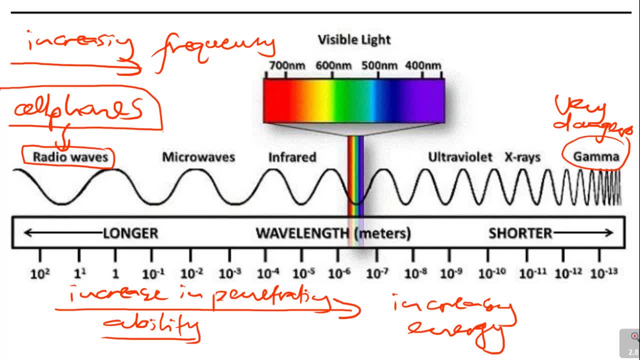 house. yes, that's your house. When you go to the house, you enter that kitchen. There are two ways. you are hungry and you want to eat. There are two different gadgets you're going to use. It's either you choose the stove or you choose to warm your food with the what With the microwave, But you're 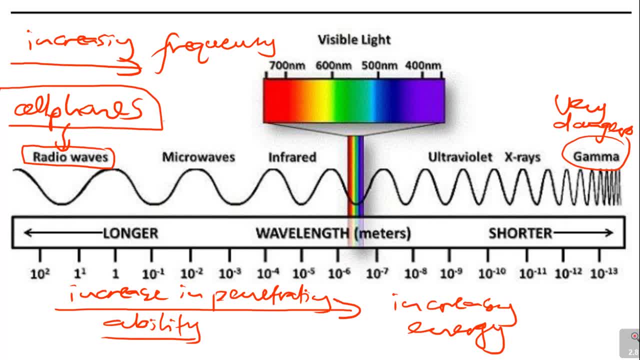 very hungry and you want to warm it fast. You know you want to cook those noodles fast Or you want to warm that food fast. What are you going to choose? You're going to choose the microwave. That's where you get number two. You choose your microwave over the stove, And if you 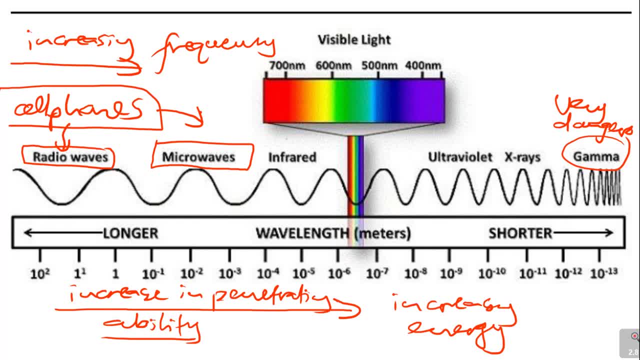 are going to cook with the stove. that is when you want to take your time, That's where you find the red part of that stove. Or you want to bake, The red part of that element gives you infrared. That red is the infrared. So let's repeat again: You are with your cell phone And what are you going? 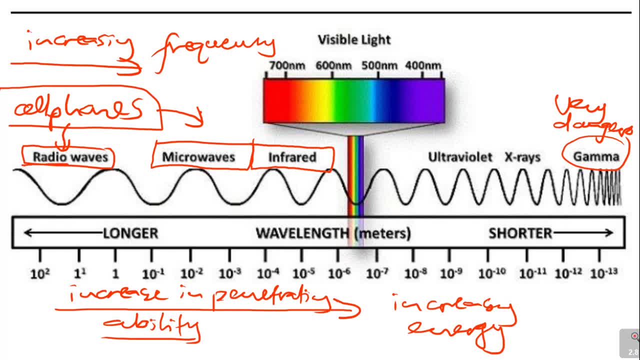 to get from your cell phone is the radio waves. From the radio wave you are hungry. from school or from work, The first thing you're going to get into the kitchen to warm your food faster is the microwave. Now, when you start cooking, you switch on your stove. Your stove turns red. Have you seen? 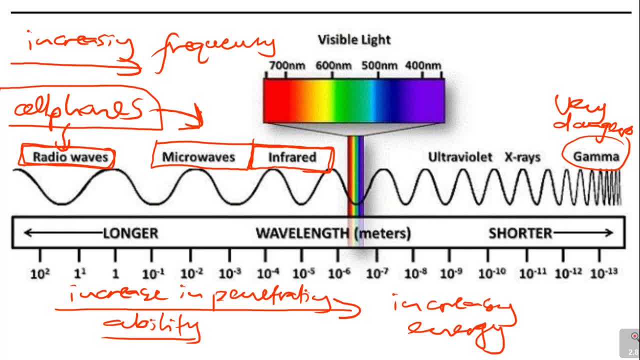 that redness in the plate, or the redness of the filament, or the rings in the oven, That stove, in baking, there is that red element that gives you the red heat. That's infrared, All right. And then you continue to say: now it's dark, You want to switch on the lights. You see, that's the light. 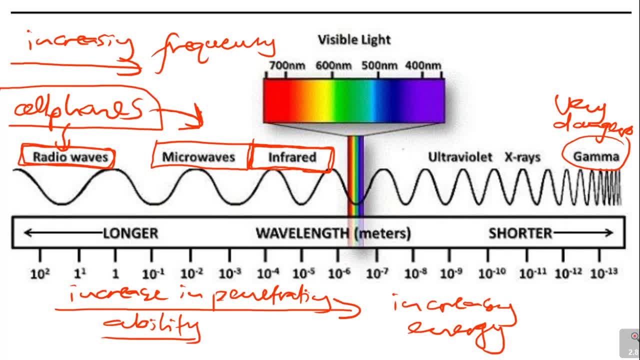 When it's dark in the house, when you're cooking, you are turning on the light. Then that's where you have the visible light. But the simpler one here is: see yourself opening up the curtains in the morning to see the sunlight. What are you needing there? You are needing, or you're. 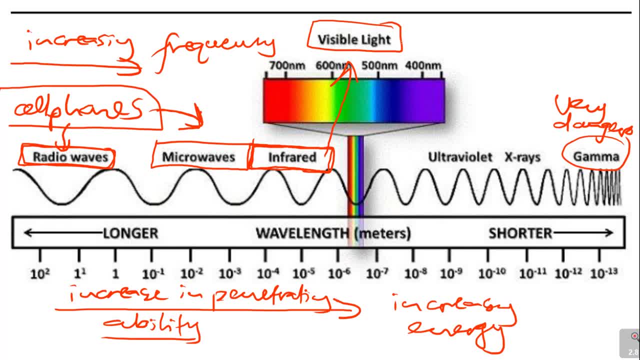 looking for the visible light, But, as they always tell you, don't stay too long in the sunlight. Don't stay too long because sunlight is dangerous. You need a sunscreen. Remember when you're going for the beach. in the beach, you need a sunscreen. What are you protecting yourself from? From UV. 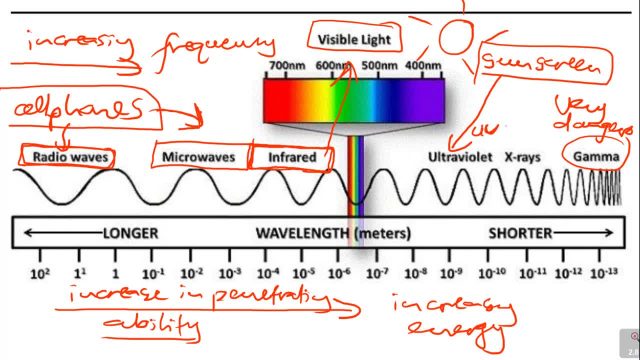 That's why it's got a UV factor of- they'll tell you- UV factor of 40. So you're protecting yourself from the ultraviolet, Are you seeing that? And then from there you go to the doctor for a checkup. You just feel yourself not fine. They say: let's take you to the. 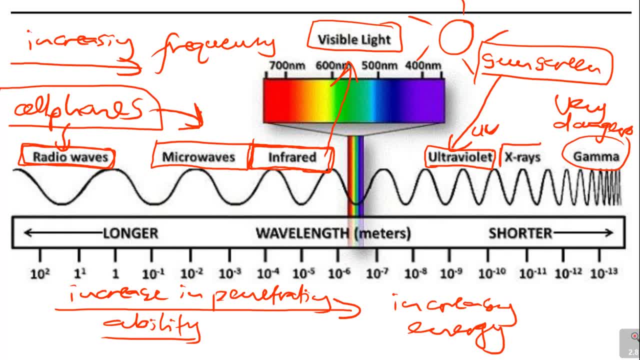 x-ray. That's where you get the x-rays, And from the x-rays, I told you, the last one is always the gamma rays. I think, as I said, I was trying to prepare, I was trying to put some images in your 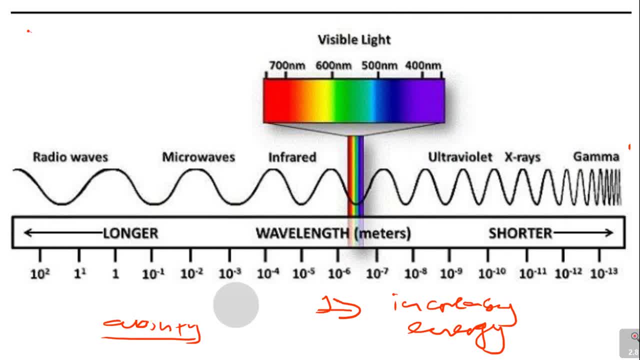 mind which need you not to sometimes use the words. If you want to use the words, it's fine, But look at this: When you're having see your cell phone, if I talk about cell phone, you you think of radio wave. If I say, go to the, 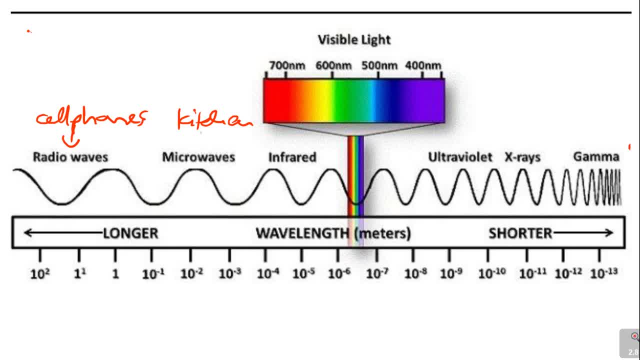 kitchen. you're going to find two things in the kitchen. You're going to find the microwave and stuff. So when you see the microwave, automatically it's the microwave. Start with the microwave, It's faster than the stuff. The stuff: give you the red part, which is the 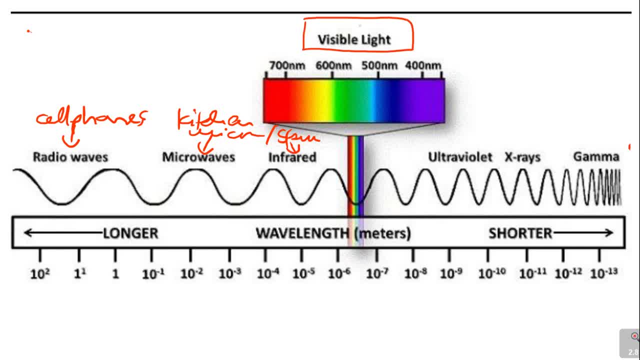 infrared And then you're opening the curtains. When you see the sunlight, what? What are you seeing? The light, That's the visible light. But be careful, protect yourself from the sun by using what? The sun protection factor, the sunscreens or the sunglasses. Why are you? 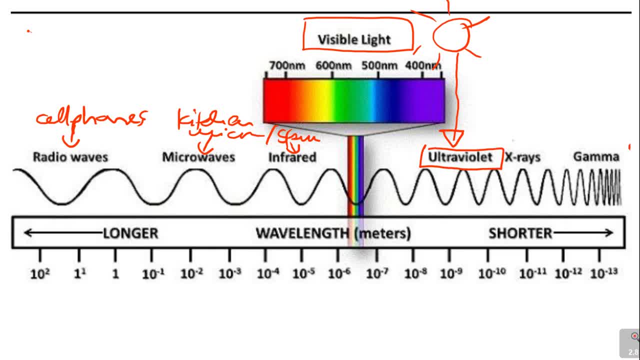 protecting yourself from ultraviolet. And then, when you go to the hospital for a checkup, what are they checking up? They use the x-rays and the dangerous one is gamma rays. So the moment the cell phones remember cell phones. you are safe with the cell phone side, but you are very 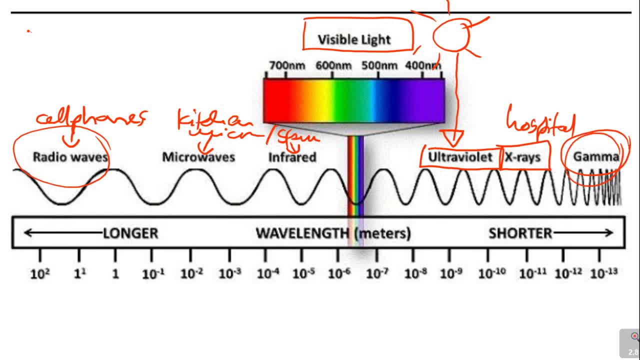 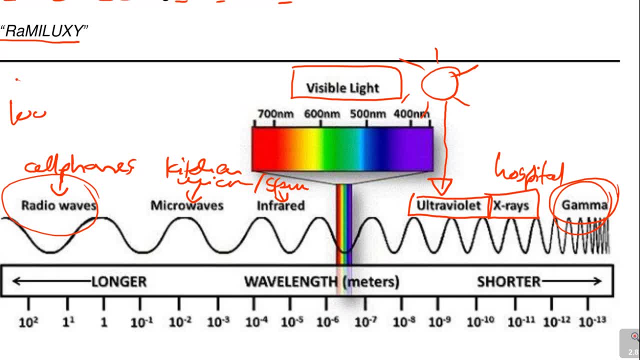 very dangerous with the camera. Those are the things that you can use, guys. Whatever case, you need to master the sequence. Either you start from radio- low penetration- Remember they wanted to do that low penetration- and to gamma it's high penetration. So it's up to you how you want to start, If you start. 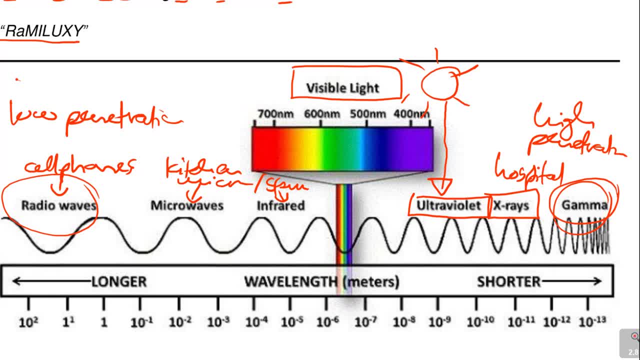 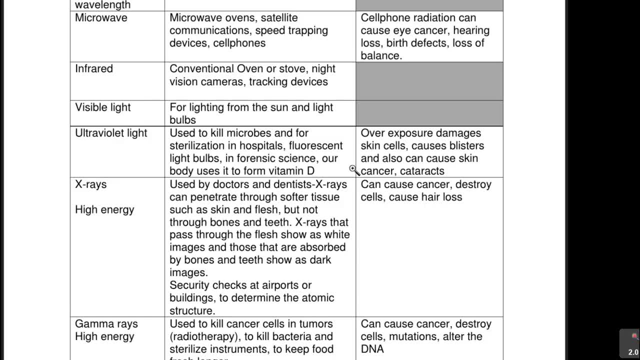 from gamma rays. you must know from high penetration to low penetration, The questions. they play around that a lot. All right, So let's move on here. The next thing. it's a summary, but your books are going to give you more information in. 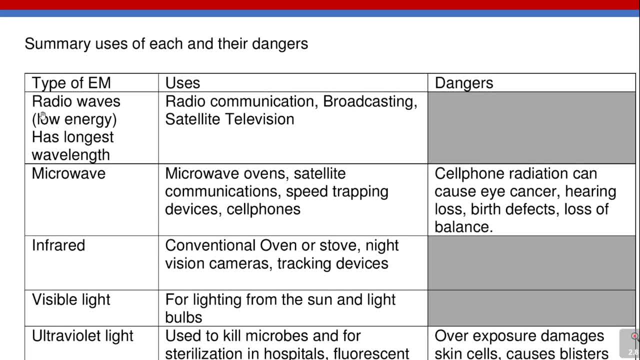 your textbook, But these are the summaries you need to know. whenever they talk of these Radio waves, we said they are low energy waves. They have the longest wavelength. This is the order. So that's your number one radio wave Uses. they will need to know for radio. 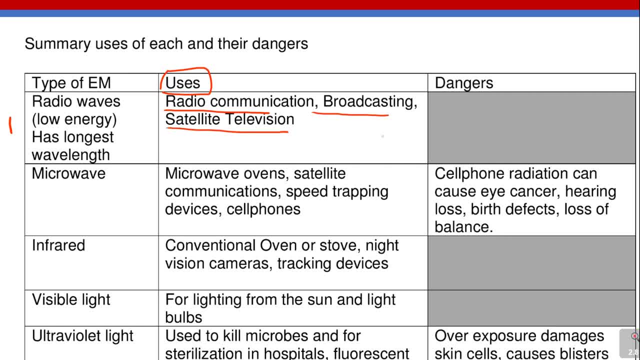 communication broadcasting satellite television Dangers. let's leave it there for now. Microwave, the microwave ovens. you find them there for satellite communications, for speed trapping devices, when they are police are using the traffic, police are using that. as for speed, 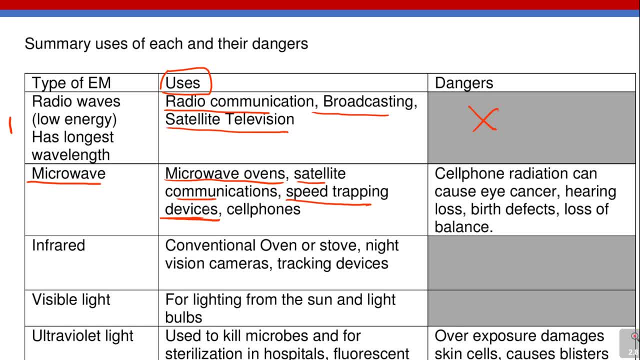 for overspeeding If you want to check that you're overspeeding. they use these microwaves Also used in cell phones, Those cell phone towers. they use the microwave, So they use it in dangers. They always talk about cell phone radiation, but we're going to look at. 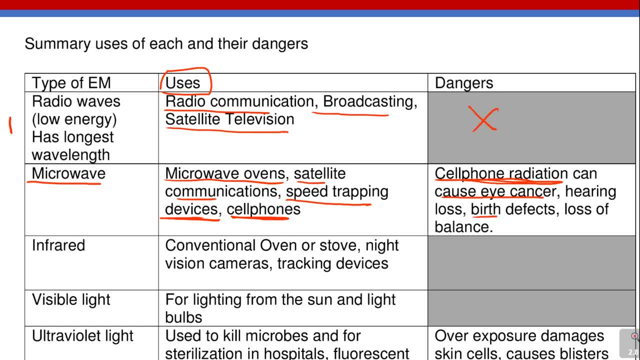 it later, which can cause eye cancer, hearing loss, birth defects and loss of balance And then. so this is dangers that they will also ask you in general. So they will ask you microwaves- where do we use them Or what do we benefit from them? And then infrared. 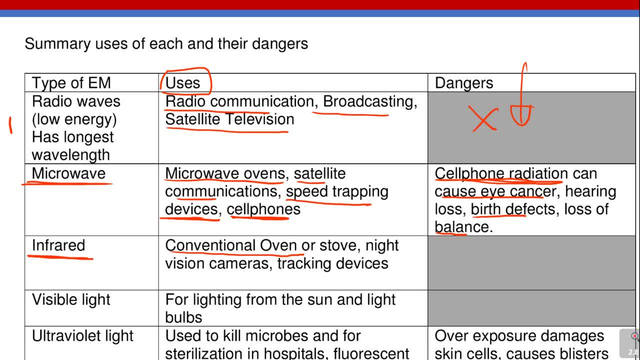 where do you use infrared For the conventional ovens? I told you that redness in the stuff is the microwave And the night vision cameras they use microwave and for tracking devices. What about the dangers? Of course, in general you can get burned, you know, and stuff can. 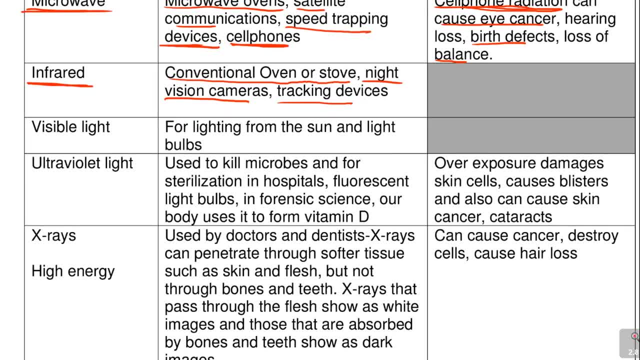 burn you Visible light. Visible light: we benefit from the normal lighting, from the sun, so that we can see from dark. I mean from darkness to light. you know for the normal lighting and we see lighting or we use it also in the lighting part: Ultraviolet. 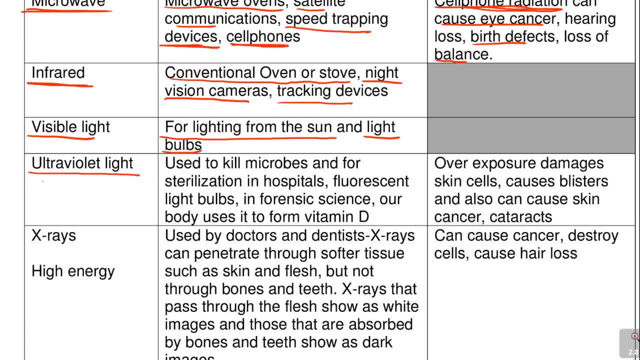 light. This is where things start getting dangerous. now They become penetrating. This is low energy. This now become high energy. They start the high energy waves, So they are used. you see, they are now used to kill microbes. Now the 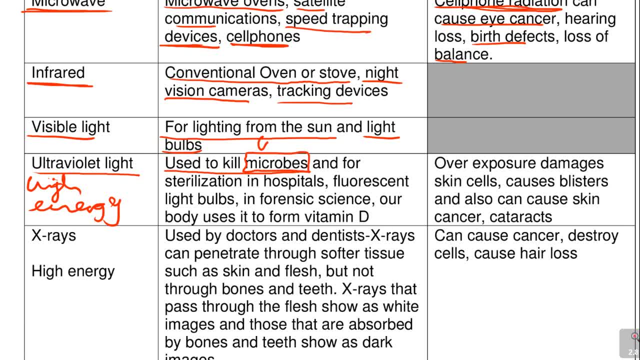 word microbes they. you just think of things like bacteria, viruses, fungi. you know bacteria, the viruses, the fungi, the germs. You know anything that is not needed, especially in a hospital. So they are used to kill microbes. 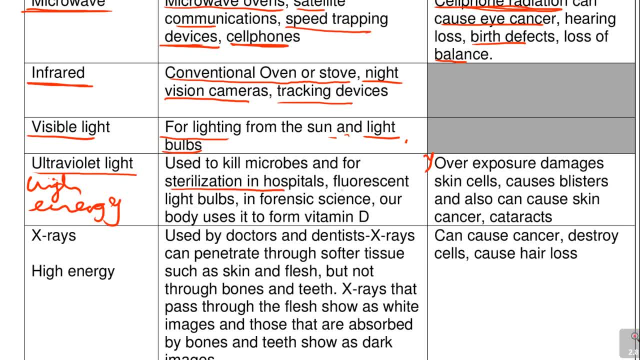 and for sterilization in hospitals. They are also used in fluorescent light bulbs, the ones that you use in the house, Those energy, energy servo lights. they use it in forensic science And then our body also uses it to form vitamin D. You know, there is one disease. 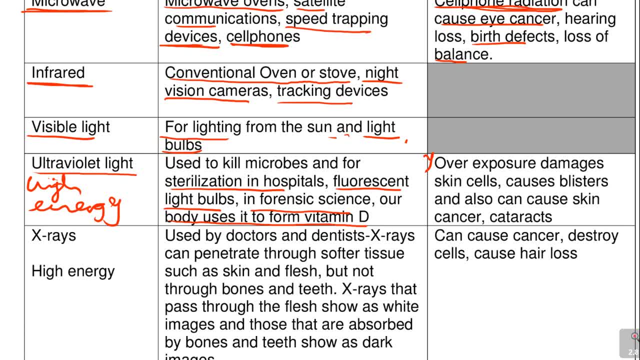 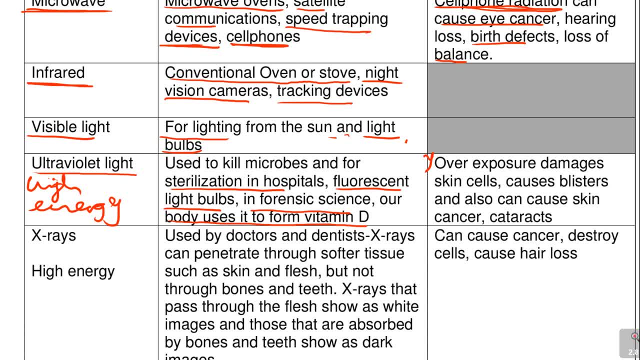 They are put in a low concentration of UV so that it can kill the jaundice, and then they can. the body then would be needing vitamin D. Now look at the dangers. Overexposure can damage skin cells. That's why you need some. 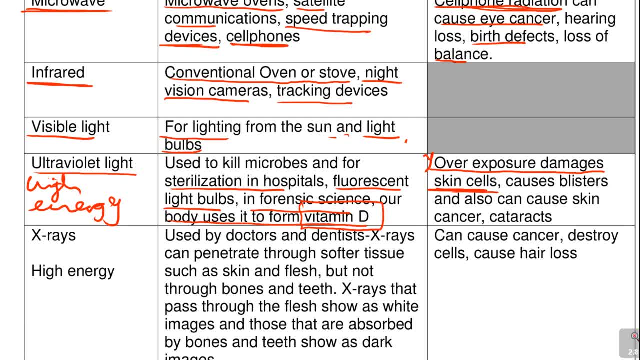 UV protectors like the sunscreens or the sun glasses. It can cause blisters and also can cause skin cancer. That's why also, it is important to to protect your eyes so that they don't cause cataracts, and it can also cause uh. 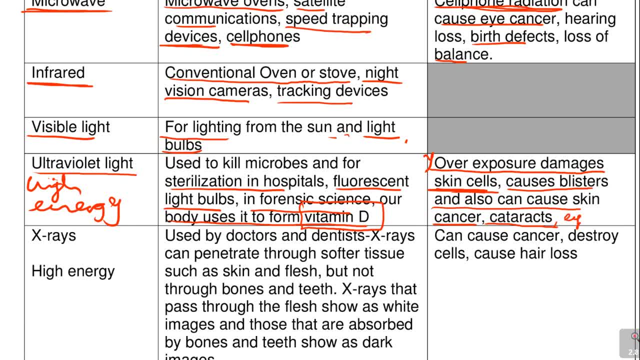 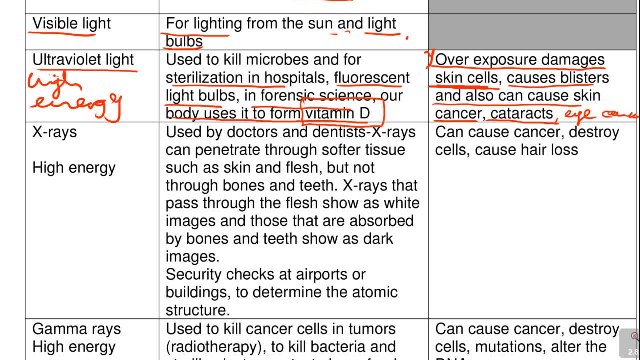 in there. it can cause eye cancer. you know eye cancer. this is the uv. you need to be careful of the uv light. that's why you can't look directly into the sun. x-rays: these are high energy, again used by doctors and dentists. x-rays can penetrate through the softer tissue as such as the skin. 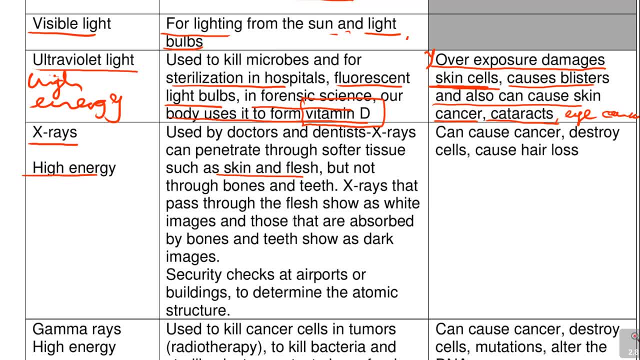 flesh but not through the bones and teeth. x-rays that pass through the flesh show as white images, and those that are absorbed by the bones and teeth they show as dark images. so that's how they check if you have a broken bone or you've got a fractured bone and like that, and then also x-rays. 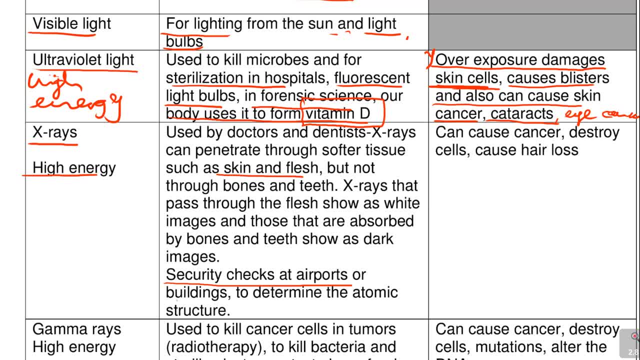 are used as security checks at airports or in buildings. to determine is also used to determine the atomic structure. so when you talk about x-rays, don't forget number one: they're used by doctors and dentists, the hospitals. two, they're used at security checks in airports. that's why, whenever they check in, 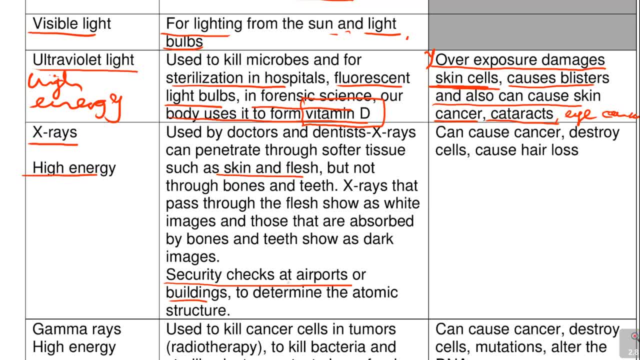 buildings to say, guns are not allowed. they put your bag through a certain machine that is an x-ray machine that checks what is inside your bag. you know. but they are dangerous. they can cause what. they can cause cancer. they can destroy cells. too much exposure can destroy cells and can cause hell. 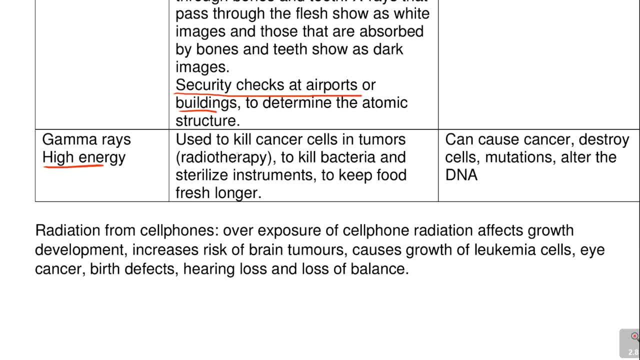 gamma rays. these are high energy rays. they used to kill also cancer cells. so if you want to treat cancer cells such as tumors, they call it radiotherapy. so you say i'm going for radiotherapy, you're. they expose you to gamma rays. they also used to kill bacteria and also to sterilize. 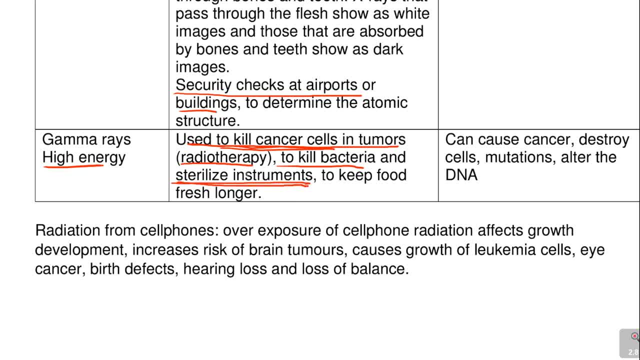 instruments, but this is not common. the most common one for sterilization, i told you, is the uv. they are also used to keep food fresh longer. now what is the dangers? they can cause cancer. in a as much as they can cure cancer, they can cause cancer. they can destroy cells. they can cause. 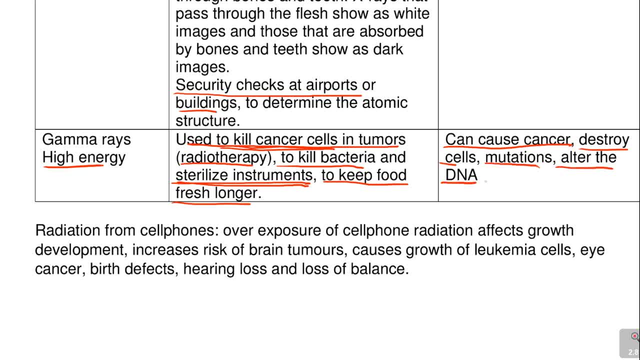 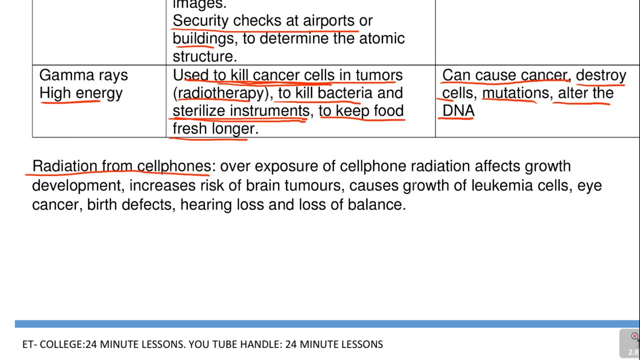 mutations. they can alter your dna or your chromosomes or your rna. they can alter this if you are doing life science. now let's look at the radiation from cell phones, also important. over. exposure to cell phone radiation affects the growth of what growth development, especially in babies, if you, they are exposed. that's why they say: when you're sleeping, don't sleep with. 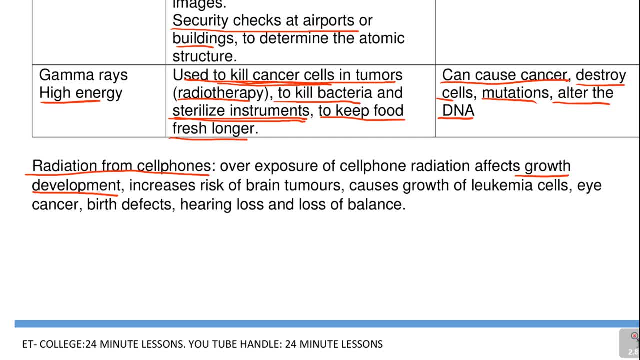 your cell phone but put it a far away from you because it's affect. it does affect growth, development, the radiation from cell phones. it increases the risk of brain tumors, it causes the growth of leukemia cells, it causes eye cancer, it causes birth defects, it causes hearing loss.